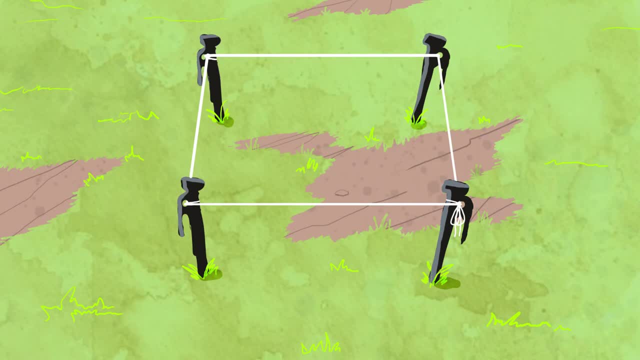 Let's dig into the soil to understand why Here is a one-foot square of soil. We'll pretend this dye is some sort of contaminant, something that might enter the environment from factories and factories. It could be debris, waste or cooling towers. 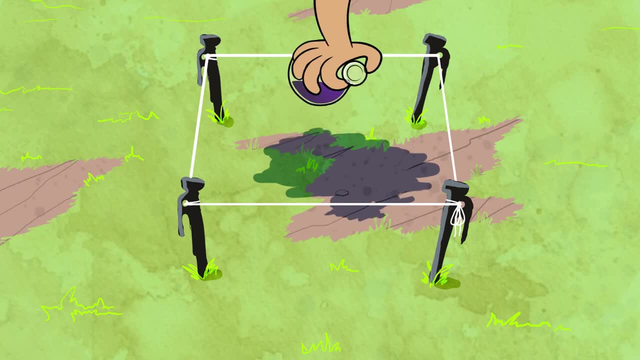 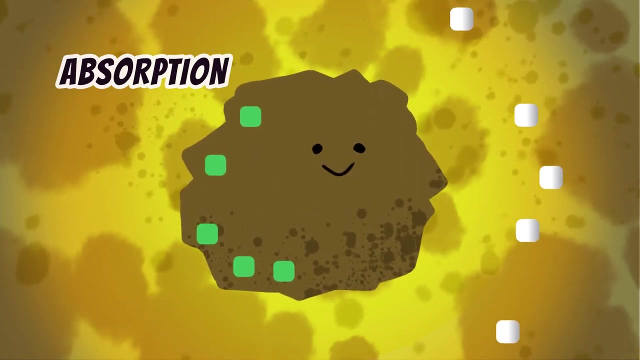 Let's pour it onto the soil to see what happens. The way this liquid enters and moves through the soil is called infiltration. As contaminants move through the soil, they undergo processes such as absorption and adsorption: being incorporated into another substance, adhering to the surface of another substance. 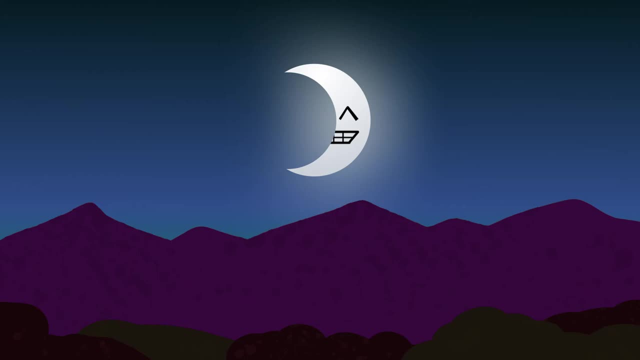 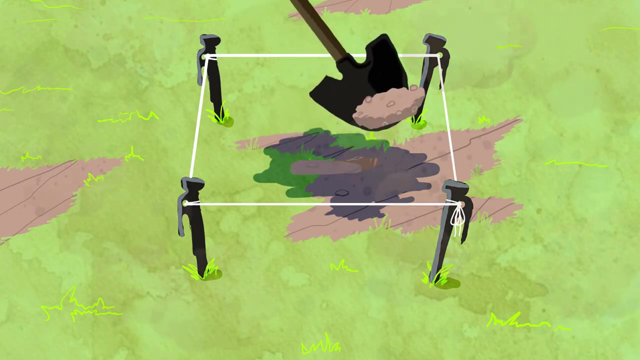 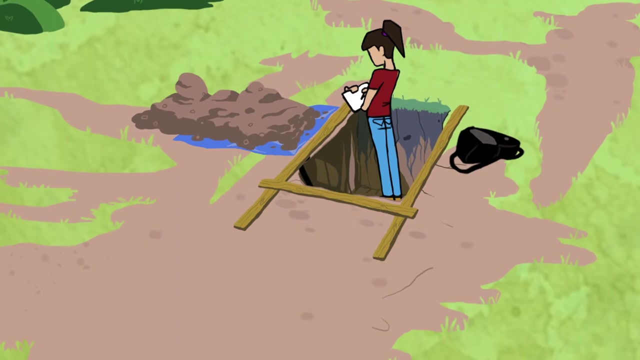 Let's wait 24 hours to let the dye percolate through the soil. Now that the dye has had time to seep down through the soil, we'll slice the soil to see what happened. Let's walk down into the soil pit. 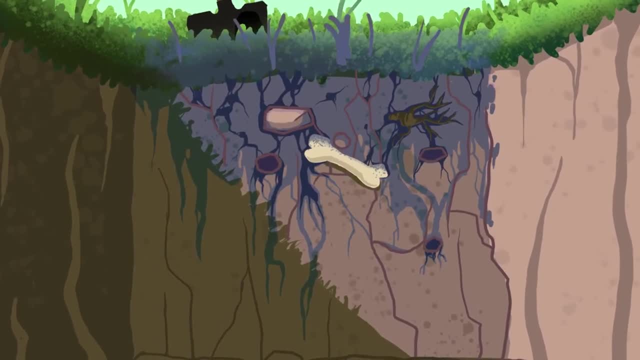 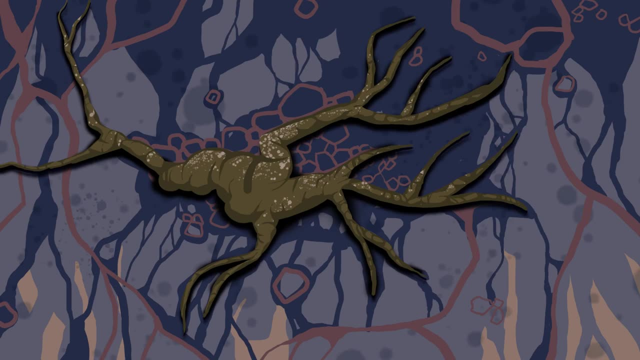 Hmm, why didn't the dye infiltrate the soil uniformly? It's easy to spot some of the reasons Here. it ran down this wormhole Over here it followed the path of a root, But we need to look at the soil microscopically. 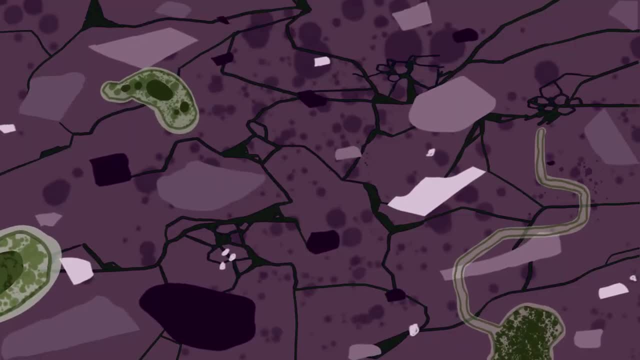 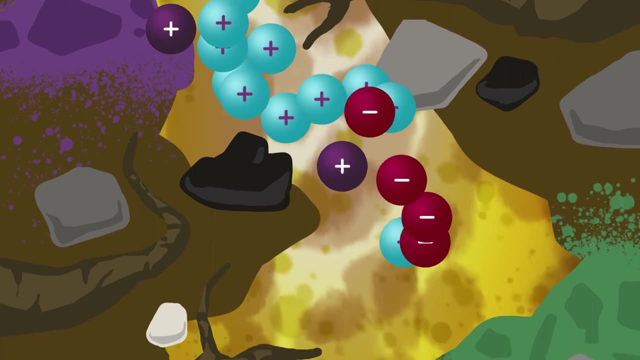 to understand some of the other flow patterns. What causes irregular adsorption? Water and contaminants act differently when they encounter physical obstructions, chemical obstructions or when things get sorbed stuck to surfaces. To learn more about that, watch our sorption animation. 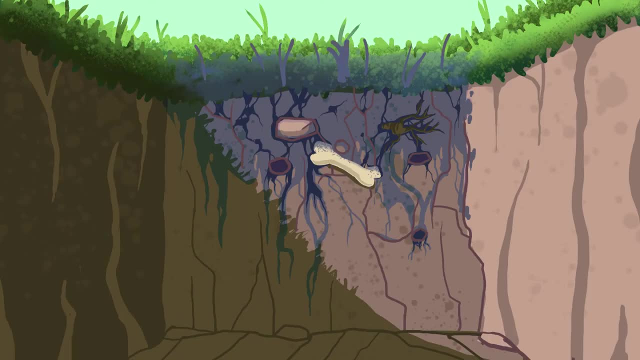 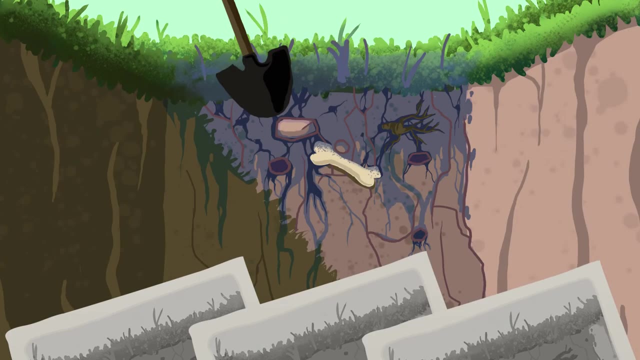 and other videos in the Science of Agriculture series. Now let's shave off an inch and look at the surface again And again And again. After comparing all of the slices, scientists can build a 3D model Showing the soil's pores. 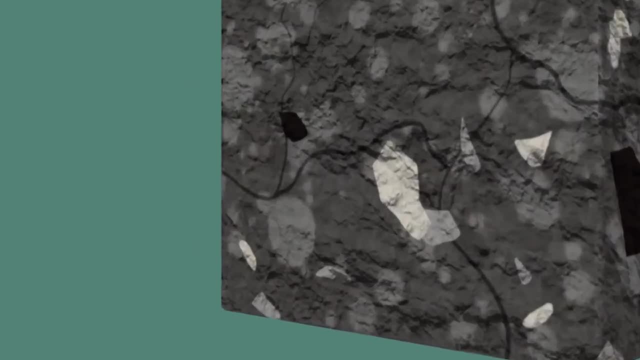 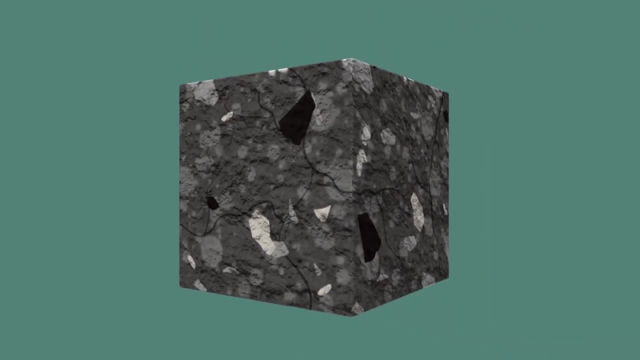 In the lab. you can do this very precisely To the cubic centimeter or even smaller. This can show you how the dye or contaminant travels through different soils By taking a large number of soil samples from many different locations and then building 3D models. 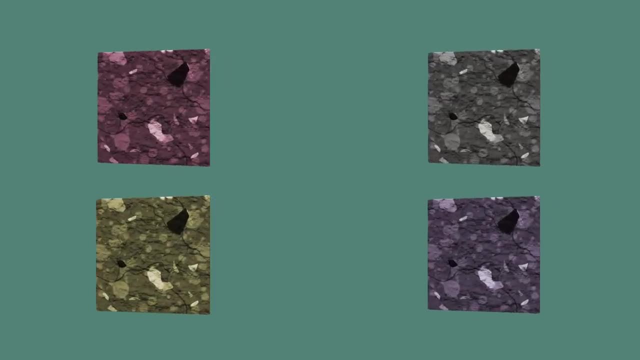 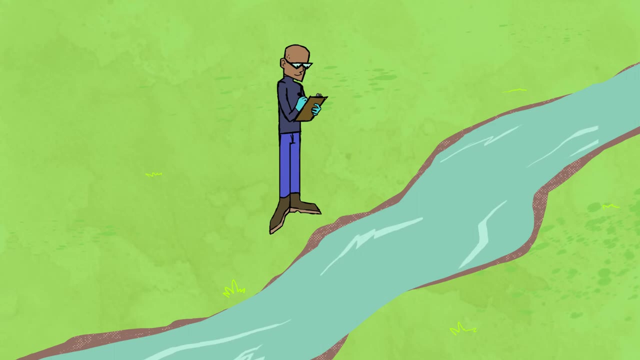 scientists have discovered that contaminants can infiltrate natural soils in complex ways. That's why, for example, when scientists try to determine whether they need to restrict use of a part of the stream, they need soil samples from the streambed in many locations.